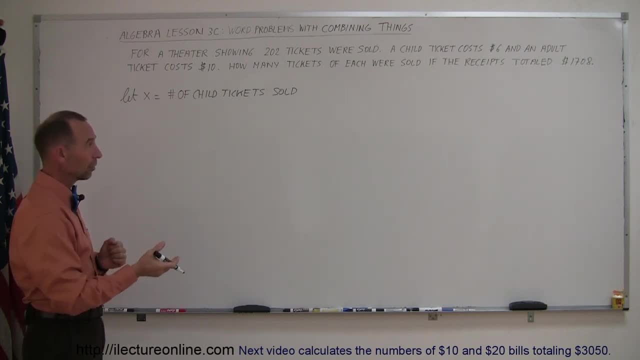 of 202 tickets. So subtract from that the number of children tickets that we end up with the number of adult tickets. So the total 202 minus the amount sold for children equals the number of adult tickets sold. Alright, now that we have that very well defined. 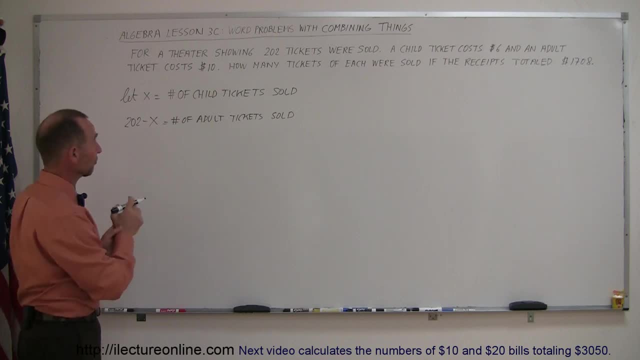 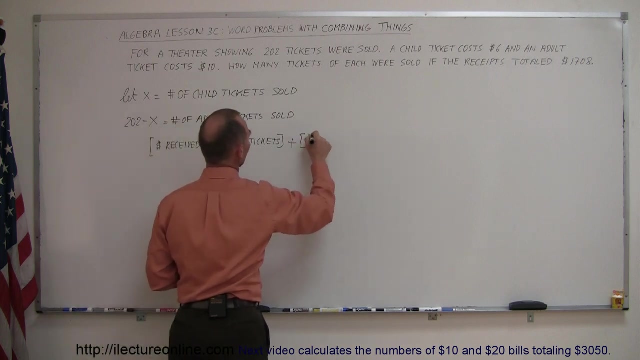 now we can go ahead and come up with an equation to help us solve the problem. We're supposed to find how many of each tickets were sold, So we can say that the dollars received for children's tickets, so the money received for child tickets plus the dollars received for adult, 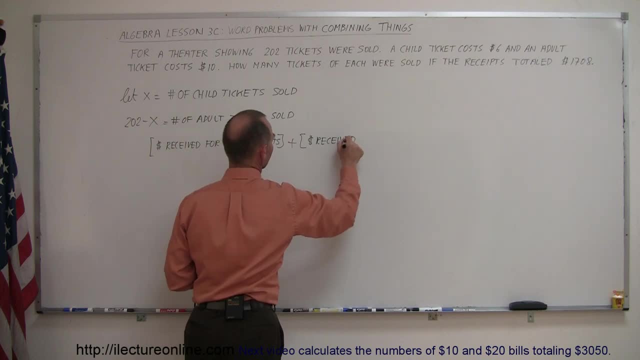 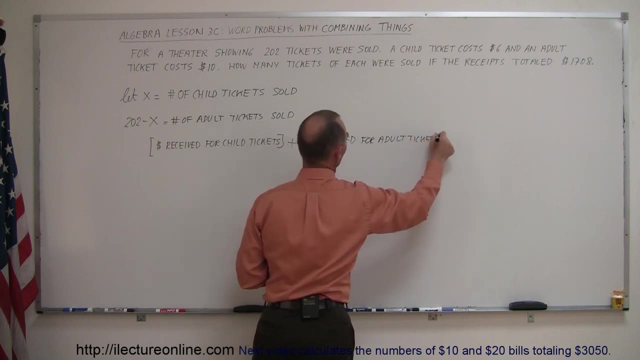 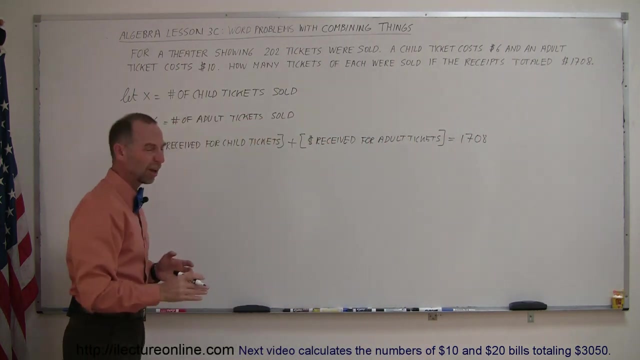 tickets must total up the total amount of money that they received, which is $1,708.. Now notice how, again, I write it out very long-handed, but again it makes sense when you do this. This is the amount of money you receive for children's tickets. 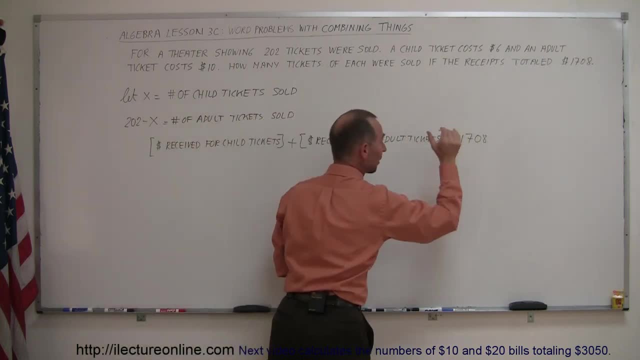 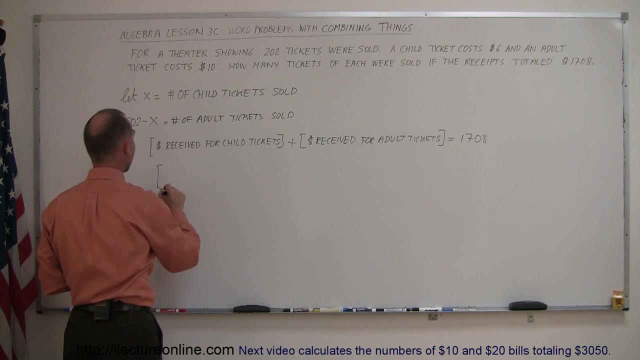 This is the amount of money you receive for adult tickets. Add them together. That should be the total amount of money you receive. Now, how do you algebraically express the number of dollars received for the child tickets? Well, you can go ahead and take the cost per ticket. 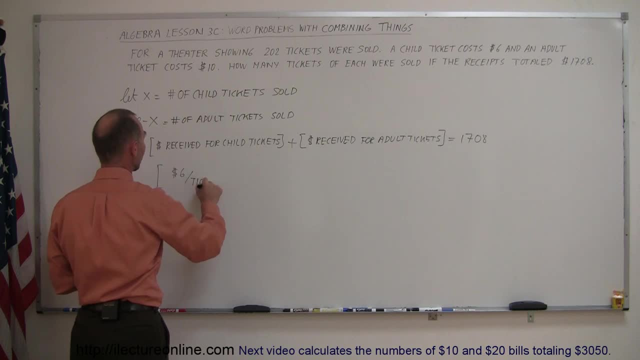 which is $6 per ticket, and you multiply that times the number of tickets. So the cost per ticket times the number of tickets gives you the total cost for all of those tickets. You do the same for the adult tickets. There we have the cost of $10 per ticket. 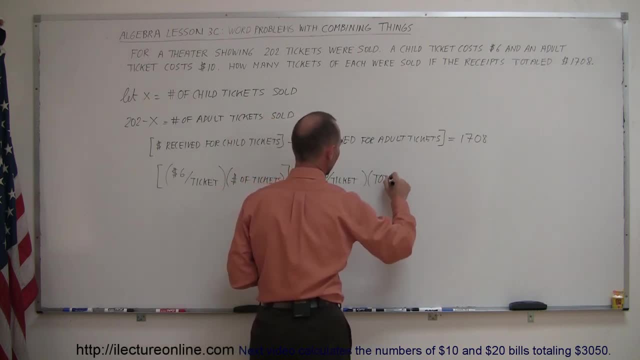 And then you multiply it. You multiply that times the total number of tickets, for the adults of course, And that should add up to $708.. Now let's write in what those are. So the numbers, the $6 per ticket. 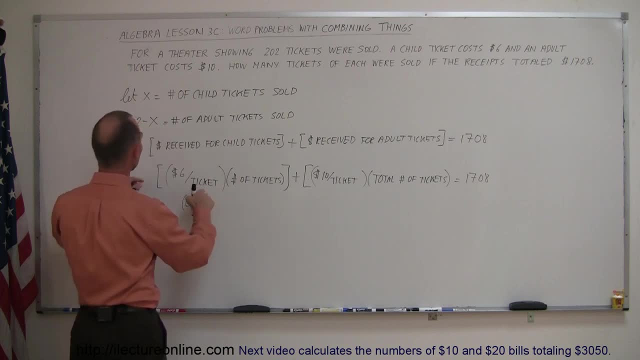 so that's 6 times the number of tickets, and these are children's tickets. the number of tickets is x, So that's the total value of all the children's tickets plus the dollar per ticket, that's 10, and multiply that. 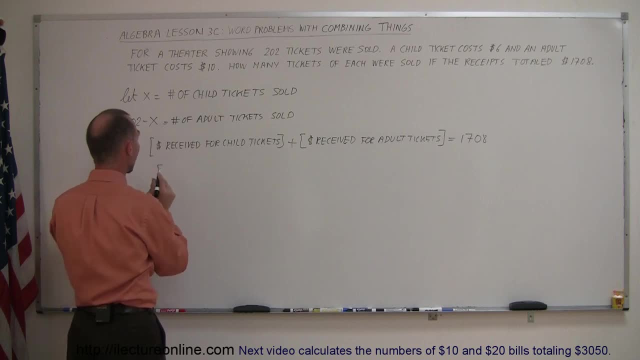 received for the child tickets. Well, you can go ahead and take the cost per ticket, which is $6 per ticket, and you multiply that times the number of tickets. So the cost per ticket times the number of tickets gives you the total cost for all of those tickets. 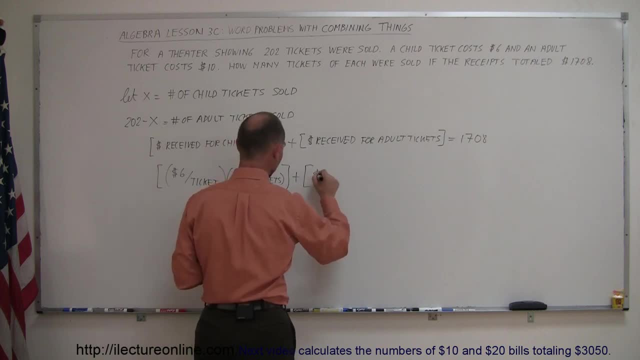 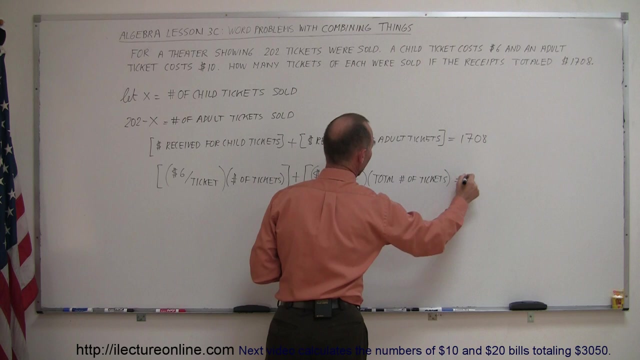 You do the same for the adult tickets. There we have the cost of $10 per ticket, And then you multiply it. You multiply that times the total number of tickets for the adults, of course, And that should add up to $708.. 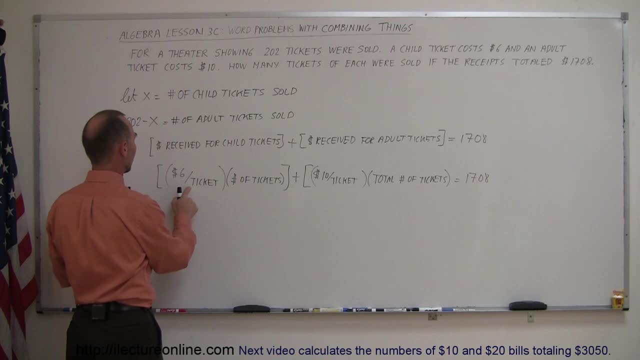 Now let's write in what those are. So the numbers: the $6 per ticket, so that's 6 times the number of tickets, and these are children's tickets. the number of tickets is x, So that's the total value of all the children's tickets. 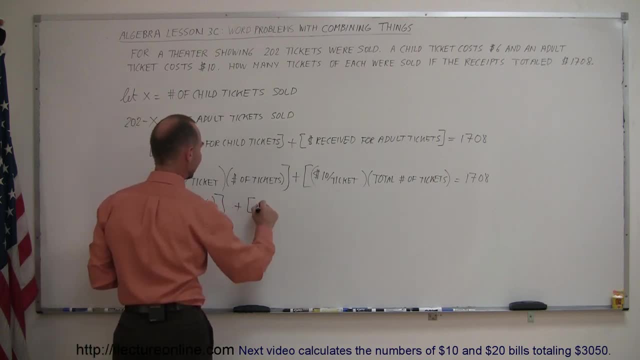 plus the dollar per ticket, that's 10, and multiply that, Multiply that times the number of tickets, which was 202 minus x for the adults, And that adds up to $1,708.. And now we're ready to solve this problem. 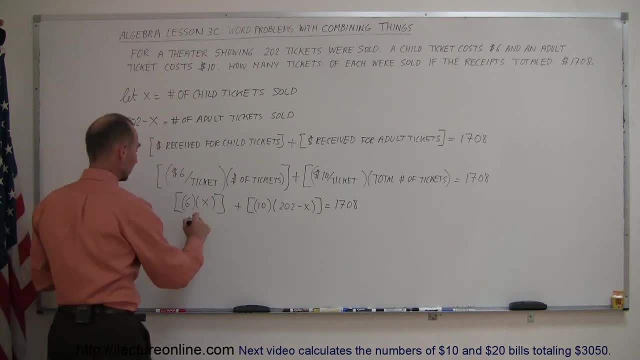 Now we're ready to solve this equation. So, simplifying things, this is: 6x plus 10 times 202 is 2,020. minus 10 times x is minus 10x, and that equals $1,708.. Now the next step is to move all the x's to one side. 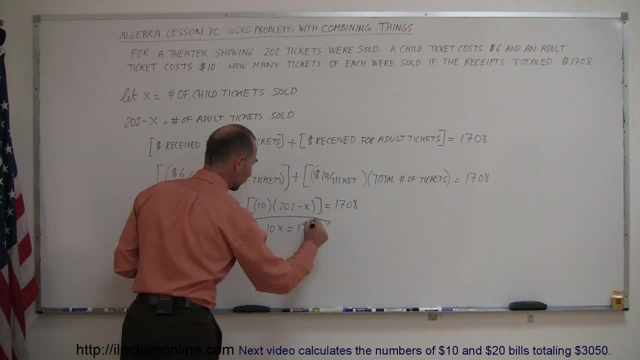 everything else to the other side and all we have to do is move the 2,020 over there. So we end up with 6x minus 10x equals 1,708 minus 2,020, because when we move the 2,020 over, 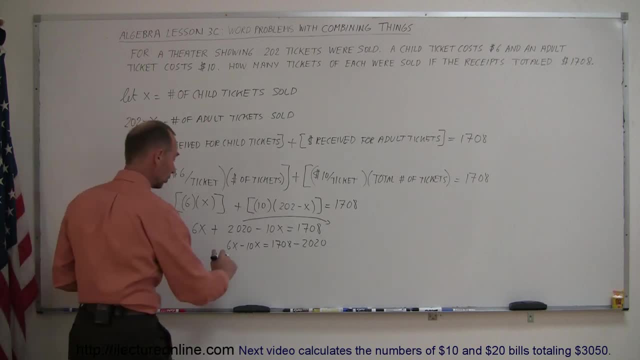 the sign changes to a negative. Now we combine like terms. So this is minus 4x. on the left side equals and that would be: hmm, the difference between this and 2,000 is 292, add another 20, that would be 312,, so minus 312. 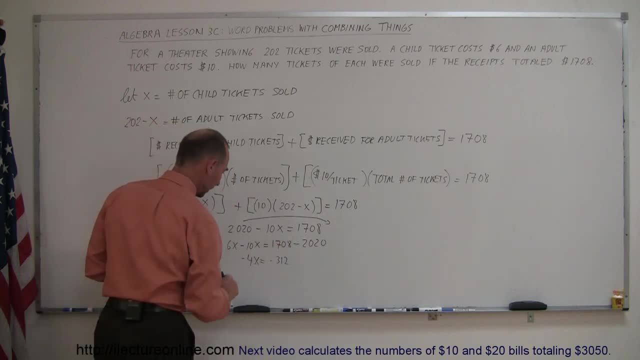 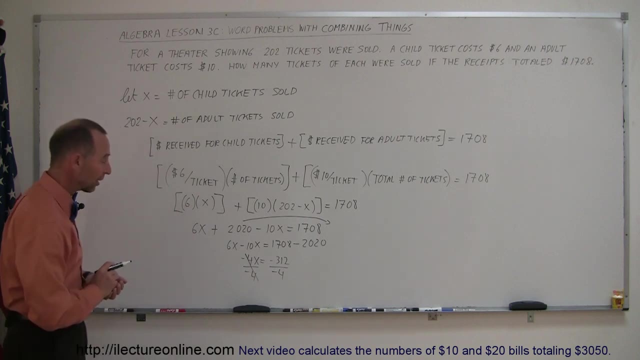 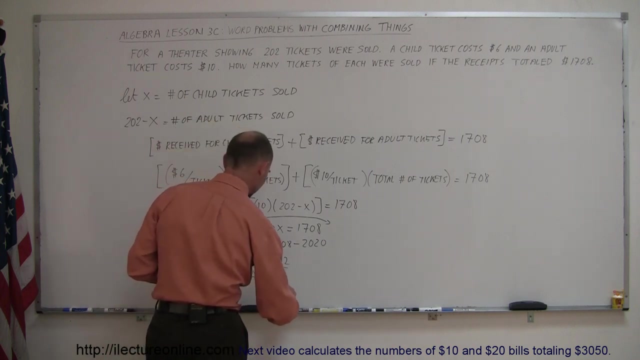 A quick check tells us that that would be correct. All right, now we divide both sides by the numerical coefficient in front of the x, so that the negative 4 cancels out. So what is 4 divided into 312?? x equals 4 goes into 31,. that would be 7 times. 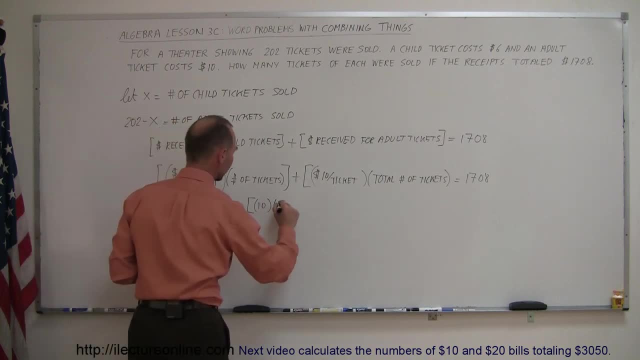 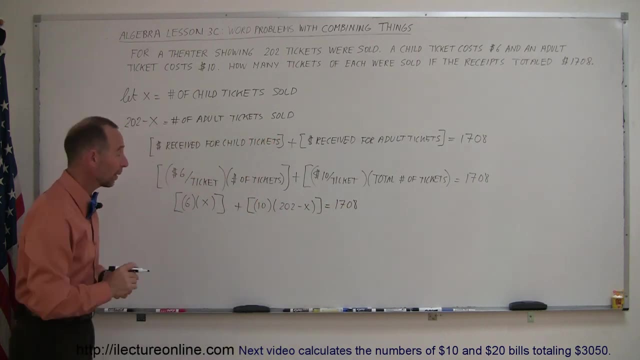 Multiply that times the number of tickets, which was 202 minus x for the adults, And that adds up to $1,708.. And now we're ready to solve this problem. Now we're ready to solve this equation. So simplifying things. 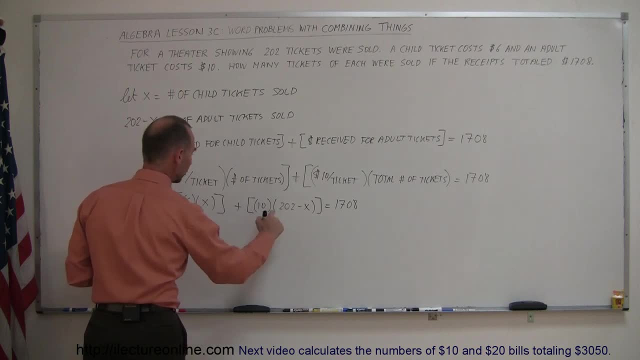 this is 6x plus 10 times 202, is 2,020. minus 10 times x is minus 10x, and that equals $1,708.. Now the next step is to move all the x's to one side. 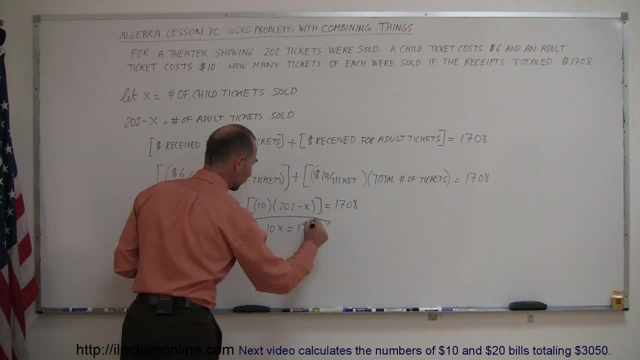 everything else to the other side and all we have to do is move the 2,020 over there. So we end up with 6x minus 10x equals 1,708 minus 2,020, because when we move the 2,020 over, 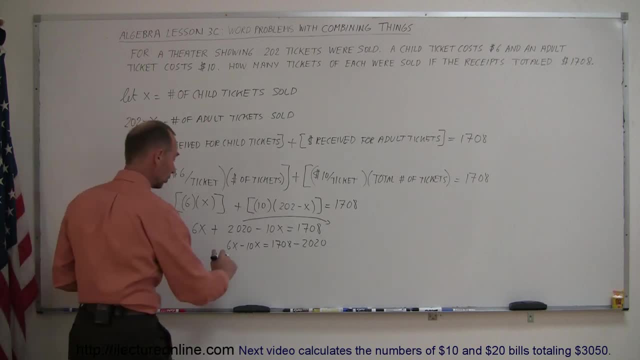 the sign changes to a negative. Now we combine like terms. So this is minus 4x. on the left side equals and that would be: hmm, the difference between this and 2,000 is 292, add another 20, that would be 312,, so minus 312. 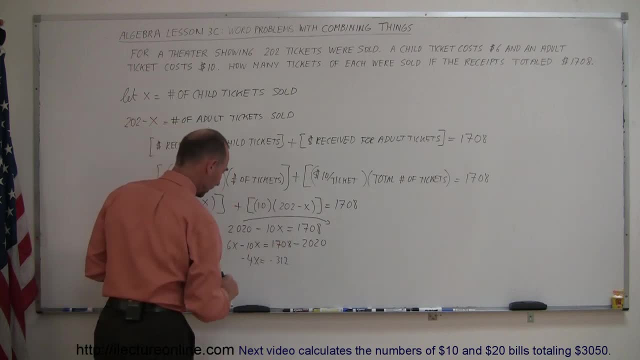 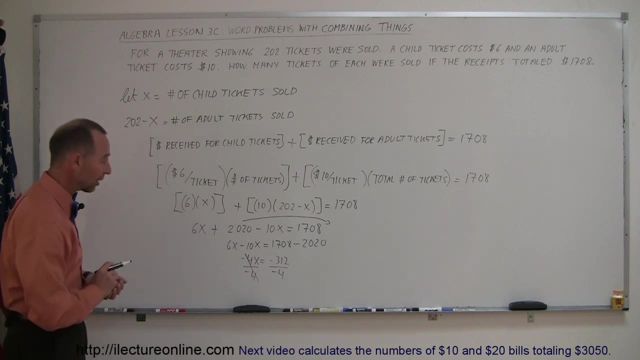 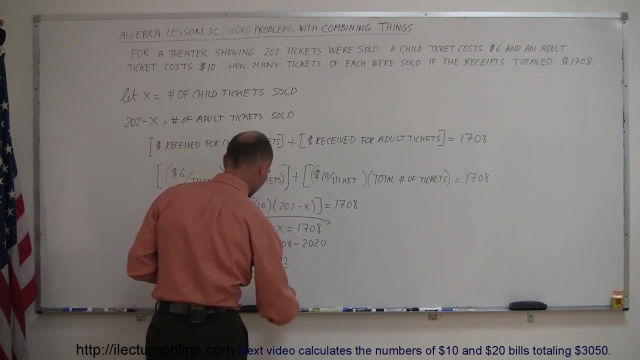 A quick check tells us that that would be correct. All right, now we divide both sides by the numerical coefficient in front of the x, so that the negative 4 cancels out. So what is 4 divided into 312?? x equals 4 goes into 31,. that would be 7 times. 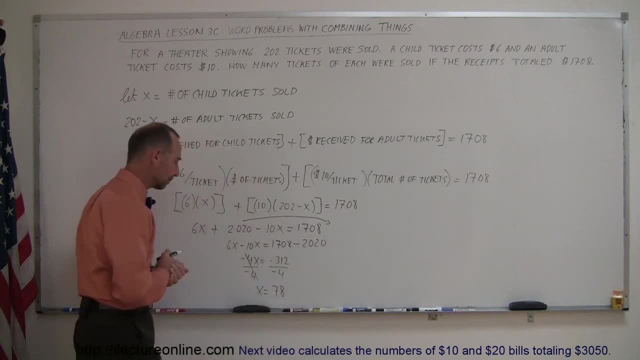 and that would be another 8.. So x equals 78. Now what does that define? What is x defined as Let's go over here? It says x is equal to the number 3.. 4 children's tickets: x is equal to 78.. 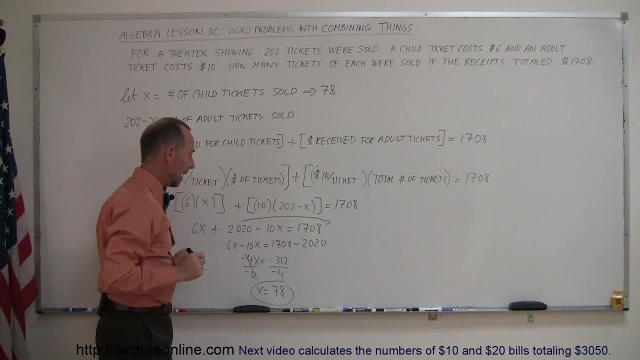 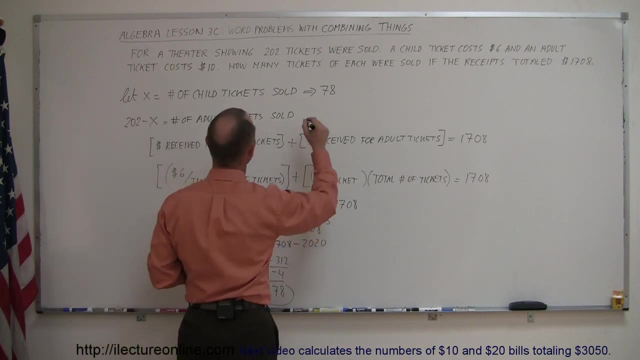 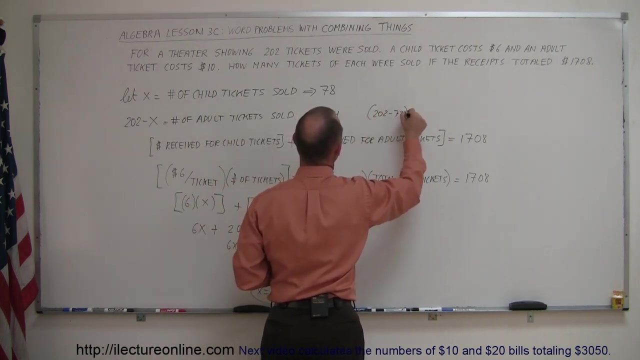 That means we sold 78 children's tickets, and if the total was 202, it would subtract 78 from that. That means 124 adult tickets were sold. So that would be the same as saying 202 minus 78, and that is indeed 124. 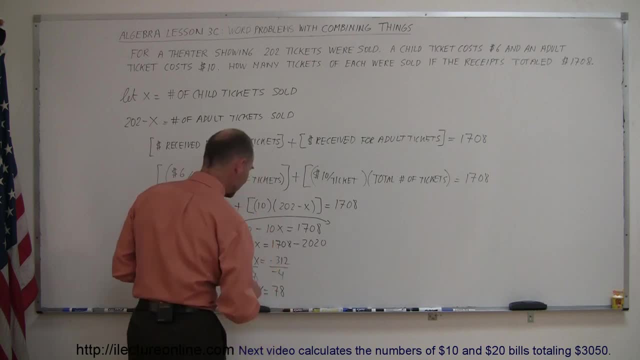 and that would be another 8, so x equals 78.. Now what does that define? What is x defined as Let's go over here? It says x is equal to the number 3.. So 4 children's tickets: x equals 78.. 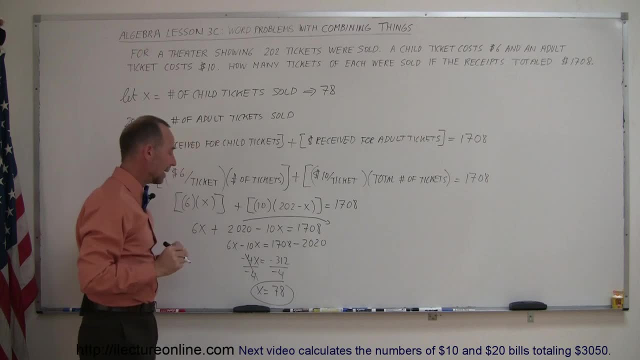 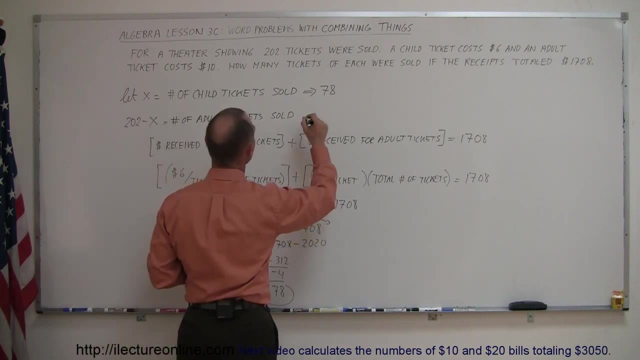 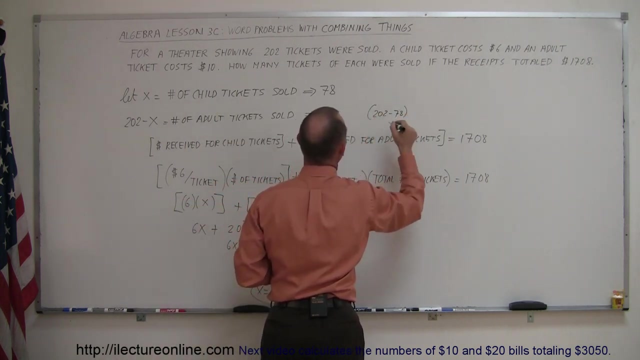 That means we sold 78 children's tickets, and if the total was 202, it would subtract 78 from that. That means 124 adult tickets were sold. So that would be the same as saying 202 minus 78, and that is indeed 124. 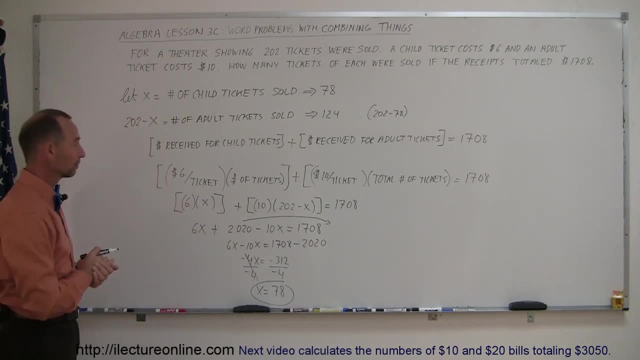 And so that's how we determine how many of these tickets were sold. All right, Let me see if I can come up with another one. Let me come up with another good example for this.